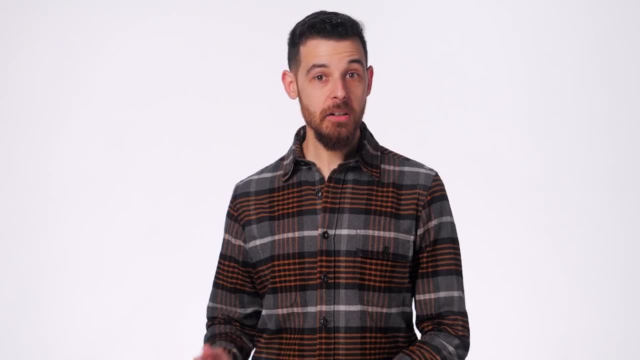 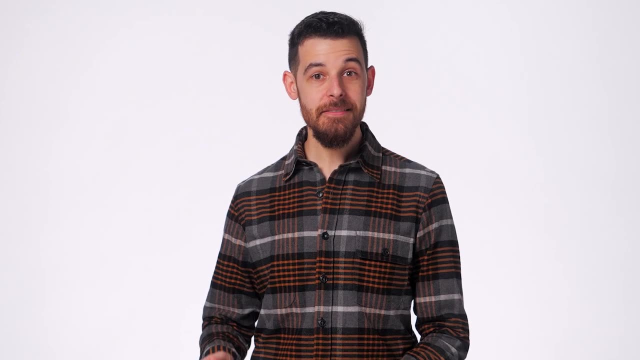 an app called Quality Xylophones. The designer on my team has come up with a new design for menus in our app and I need to build a new component for them. They've even helpfully already written the CSS for me. We can start by adding a couple of components for our menu. 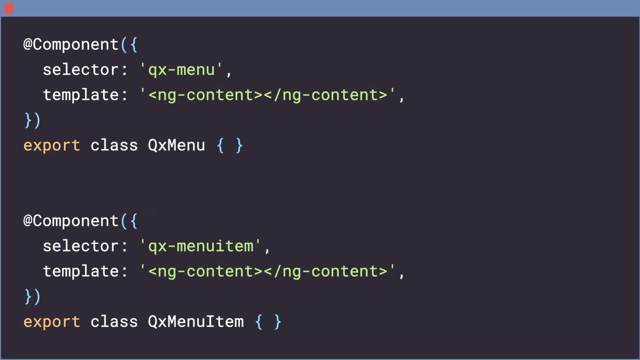 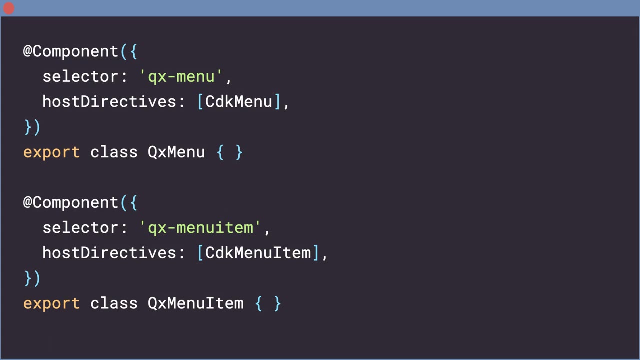 and menu item. Normally, we'd jump deep into coding out the menu functionality. now, Instead, though, we can use the Directive Composition API to pull in behaviors we need from Angular CDK. To use the new API, we add a host directives property to our components, bringing in CDK. 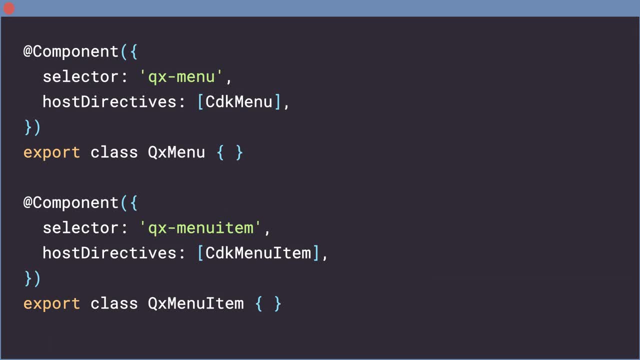 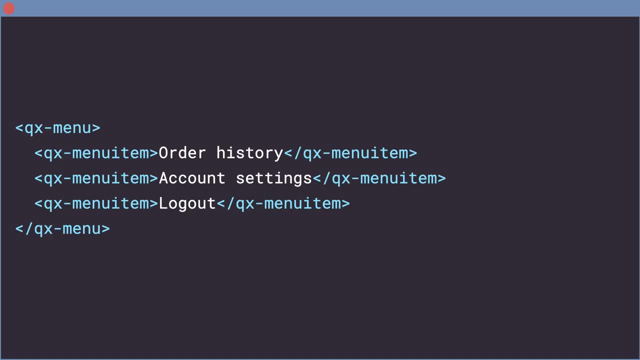 menu and CDK menu item. This will apply these directives to the host element of these components. We can try out components in the template now. Note that there's no sign of anything CDK related in the API here If we run our application. 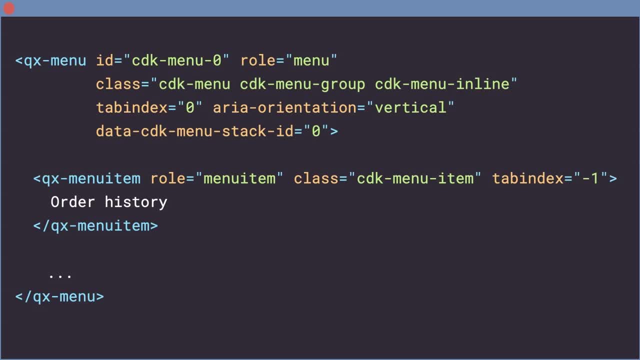 and look at the rendered DOM, we get something like this: You can see that the CDK directives have applied a number of CSS classes and attributes, so we know that the directives have been applied. We can also navigate the menu with our keyboard. It works. 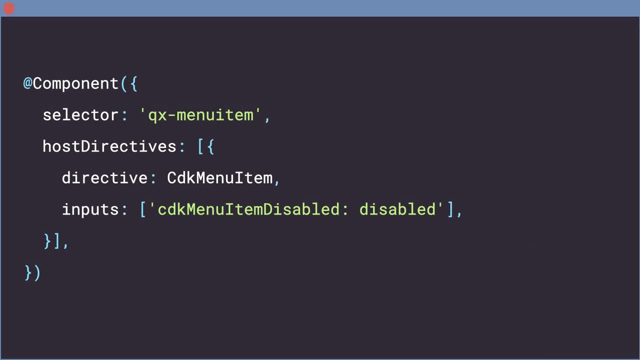 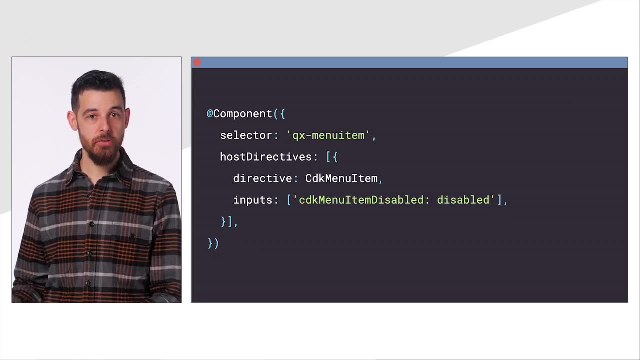 The design I'm building also includes a disabled state for the menu items. I know that CDK menu item already has an input for this, so now I can update my host directives property and expose a disabled input as part of the menu items API. 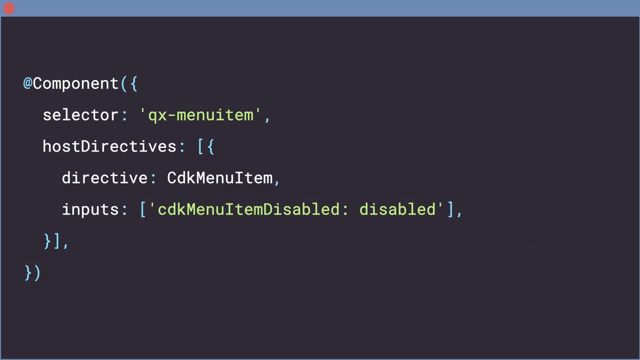 You can see, we've refactored the entry in host directives so that we can specify the inputs property. This lets us use an alias on one of the CDK menu items- inputs to be included in QX menu's public API. In this case we're aliasing the verbose CDK menu. 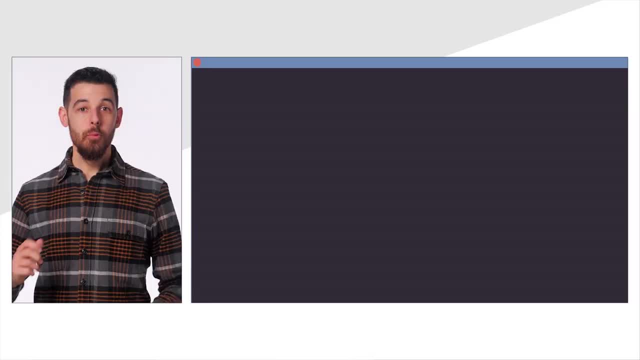 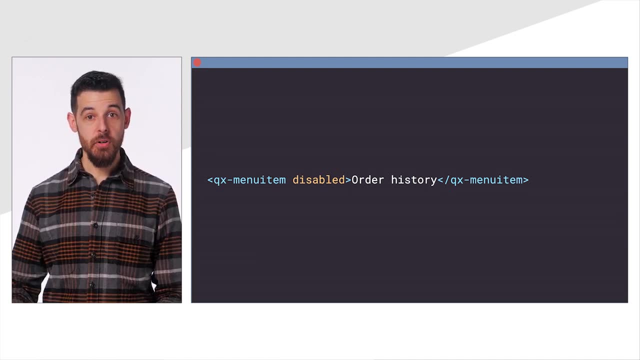 item disabled to the much shorter disabled. With this in place, we can now bind the disabled input on a menu item. You can alias any number of inputs and outputs from directives you apply in the host directives property to create a fully custom API while still delegating behavior to the composed directives.